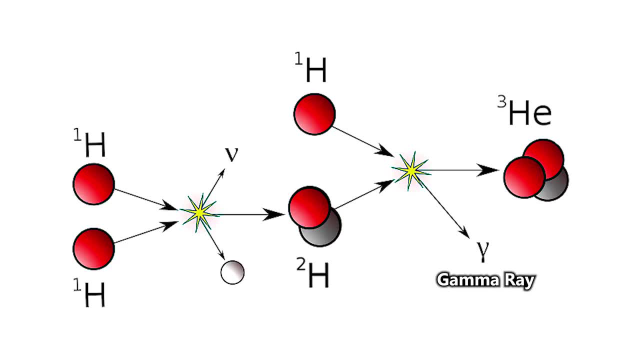 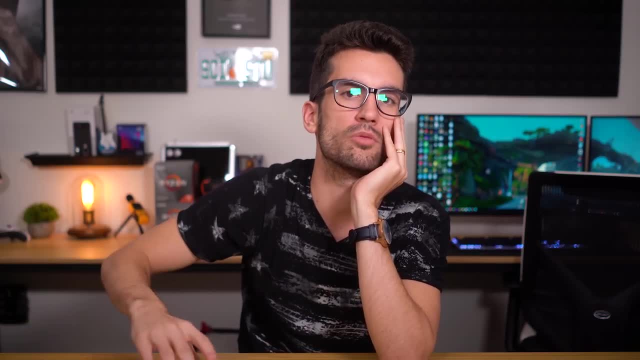 And at this point helium-3 must become helium-4, somehow. So yeah, it gets dicey. Now we're going to have to make helium-4, so we'll discuss the two most common methods. Method one involves two helium nuclei. As long as temperatures are somewhere in the range of 10 to 12 million Kelvin, they're able to smash into each other and yield helium-4, along with two protons and a ton of energy. The process takes around half a millennium to play out most of the time, which is kind of hard to fathom. 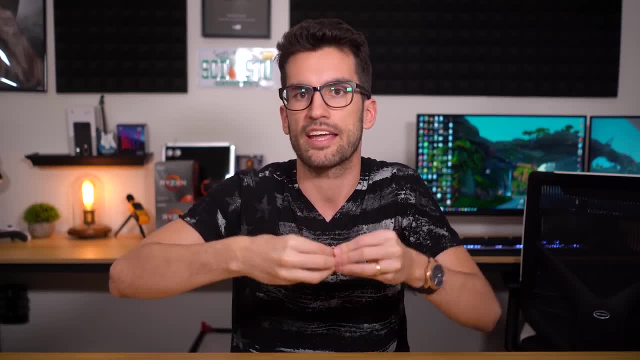 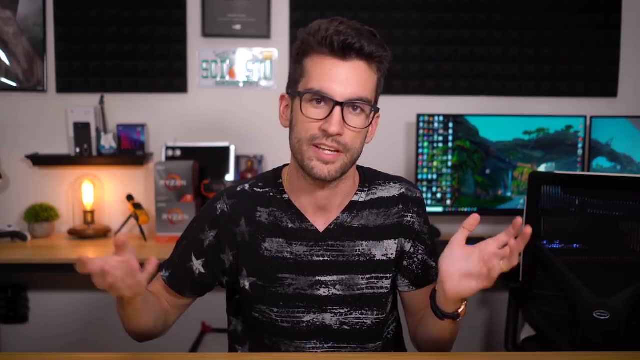 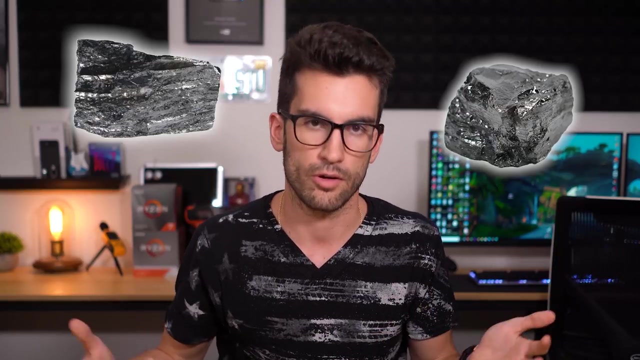 And that's because a single proton will typically smash into helium and then decay immediately And that disrupts the process between two helium atoms. And there are way more protons inside the sun And there are helium or helium atoms. So then helium-4 will go on to fuse with other smaller nuclei to form heavier elements like beryllium, carbon and oxygen. 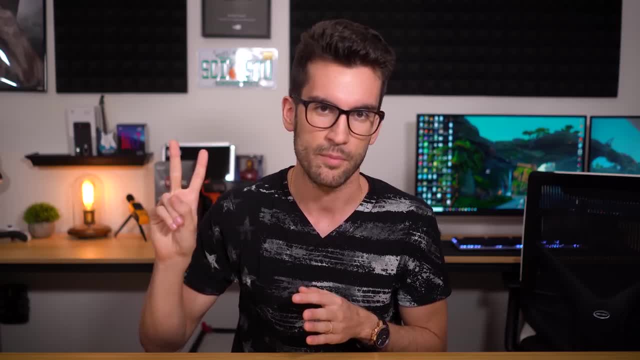 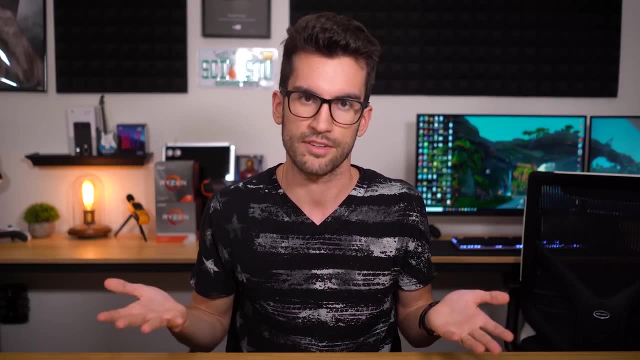 But when temperatures are much hotter, method two becomes rather common. It involves a collision of one helium-3 nucleus, that's helium, and one helium-4 nucleus, forming beryllium-7.. Beryllium-7 is interesting because it appears stable on paper. 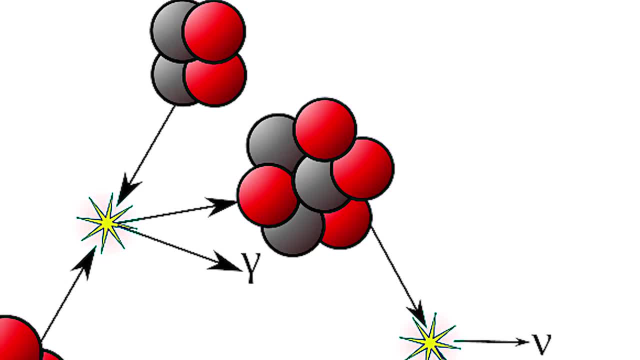 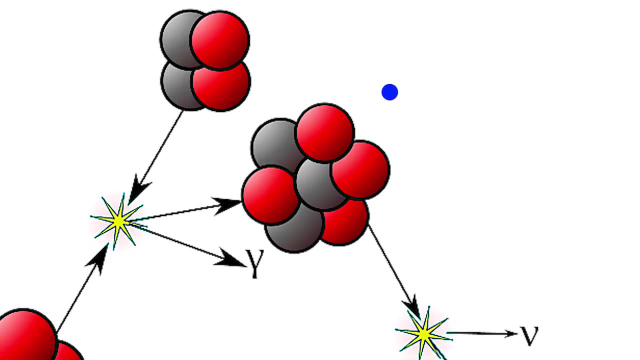 They're the same number of electrons as there are protons, But the proximities of its four protons result in something called electron capture, In which case an inner shell, or free-roaming electron, especially in the case of plasma in the sun. 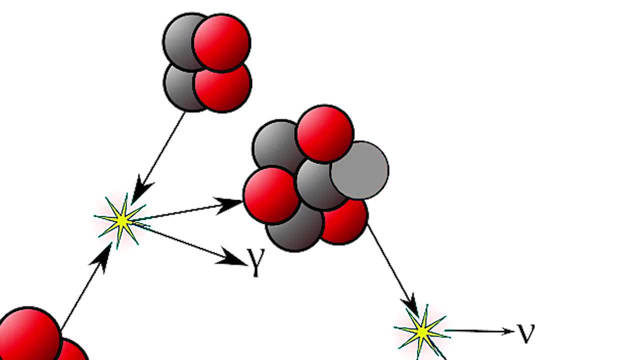 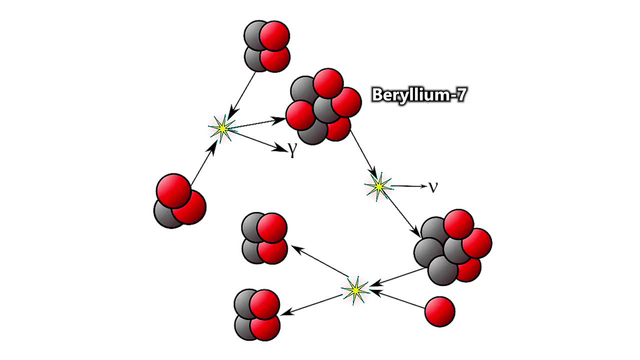 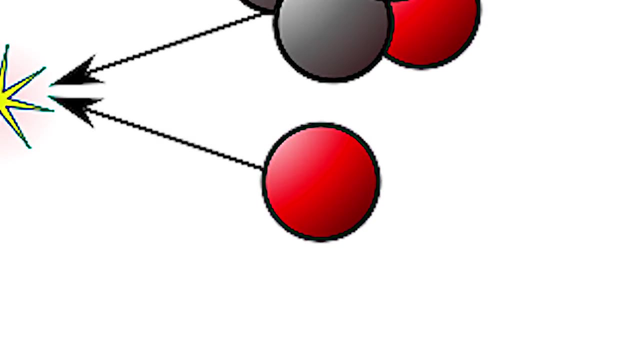 is absorbed into the nucleus, releasing a neutrino and accompanying energy. The resulting nucleus is thus comprised of four neutrons and three protons, transforming beryllium-7 into lithium-7, which is significantly more stable, Now a free-roaming proton, which there are plenty of inside the sun. 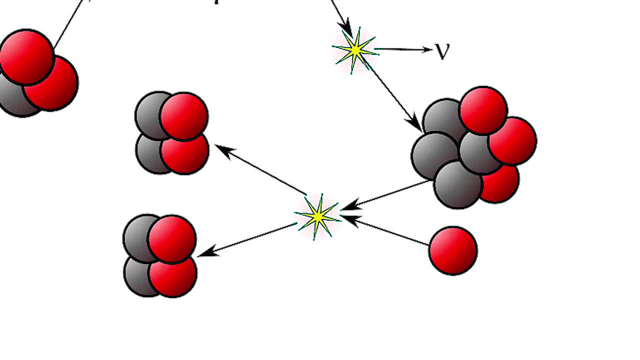 may collide with a lithium nucleus to produce beryllium, once again in a process called lithium burning, only this time with an extra neutron tucked into the nucleus, Beryllium-8,. the resultant is extremely unstable and almost immediately decays into two helium-4 nuclei. coincidentally, 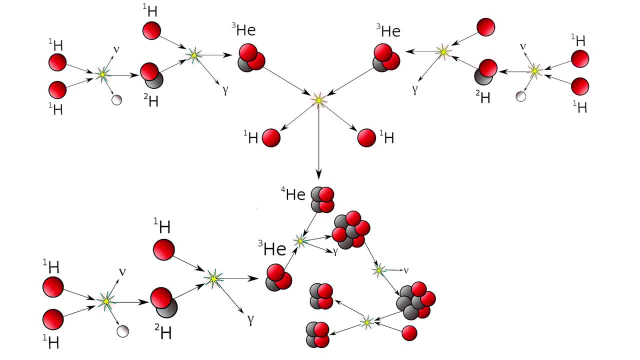 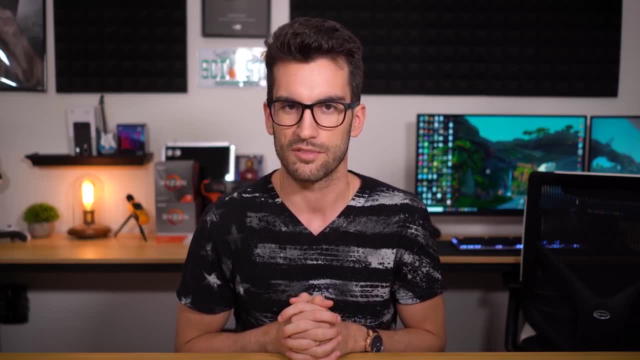 And there we go. we ended at the same place as method one, only with twice as much helium as the former. By the way, I wrote this script at 2am on a Sunday, so you'll have to excuse the more particular details I've glossed over. 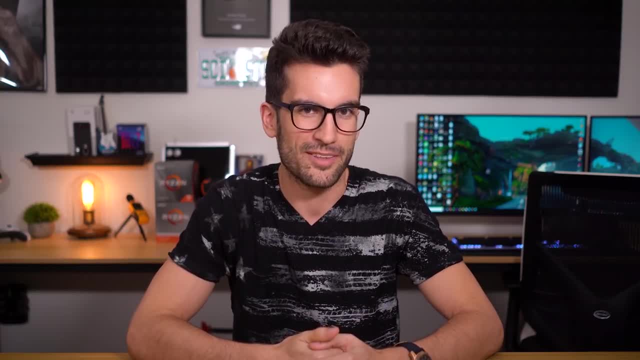 and this is a five or so minute video after all, so please be gentle with me. Thanks for the curiosity, thanks for watching and thanks for learning with us.